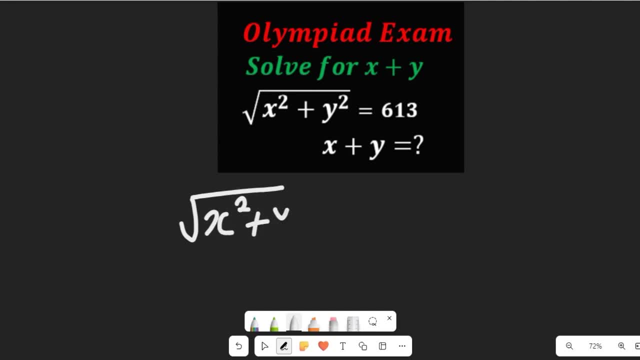 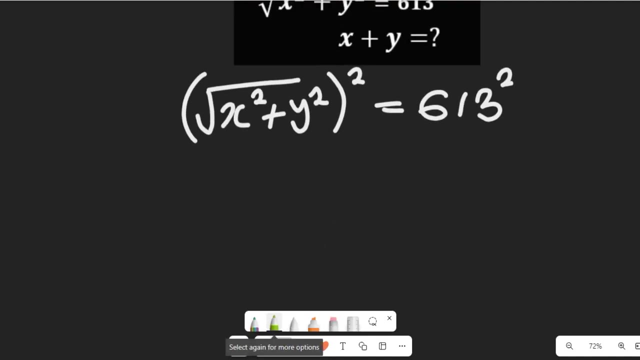 we'll have the square root of x squared plus y squared, and we're going to what? to square both sides, and this will be equal to six, one, three, all what squared. so with this expression, you'll come to see that this square will simply clear the square, and then we'll be left with x. 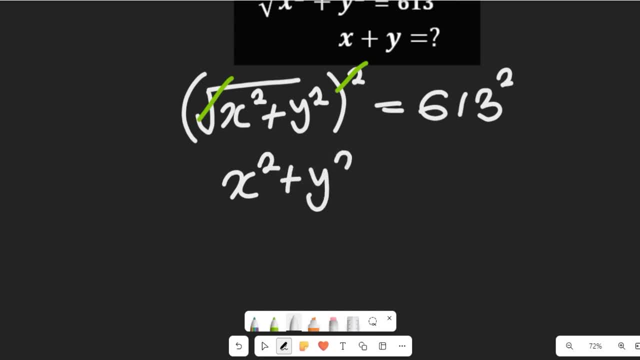 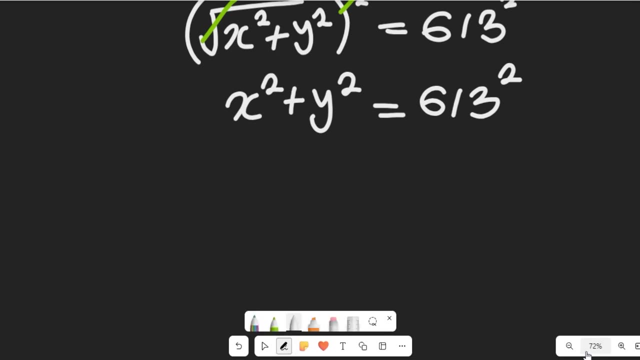 squared plus y squared, and this will be equal to six one three squared. Now let's compare this with a Pythagoras' Theorem. From Pythagoras' Theorem, you'll come to see that we have a squared and a squared plus b squared. 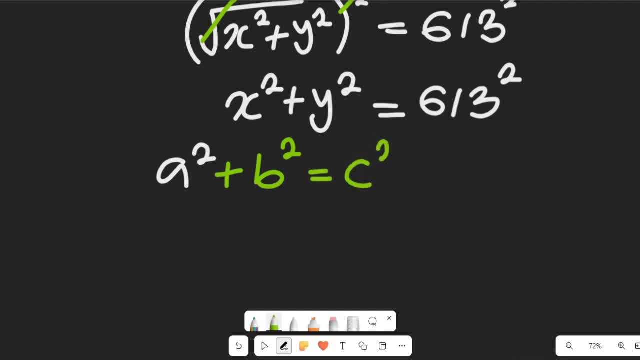 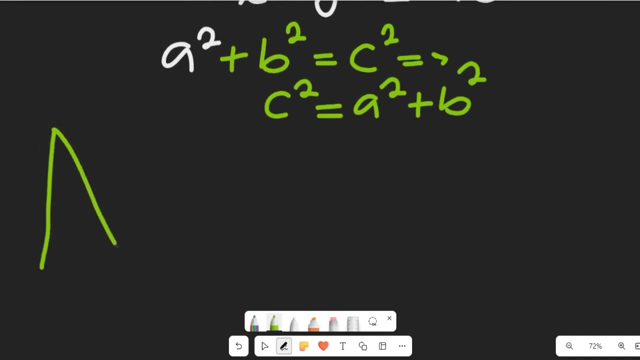 b squared is equal to c squared. or we can simply say that c squared, which is the square of the hypotenuse, is equal to the sum of the square of the other two sides. right, so if we have a triangle, if we have a triangle, let's say we have a triangle and this is a triangle, if we want to know the sides. 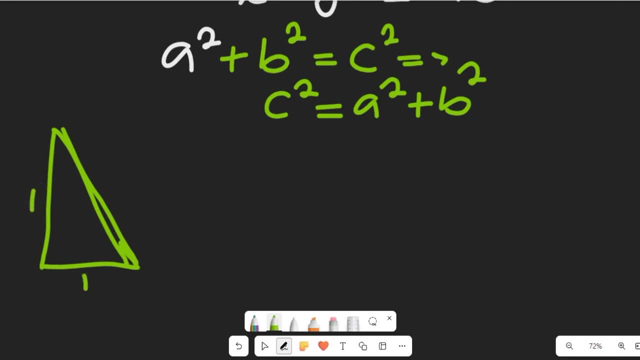 you should know that this side is one and this side is one and this other side, with this, will have this as the square root of one, because if c is equal to uh, c squared, we can get the c side to be equal to one squared plus one squared, and that means c squared will be equal to. 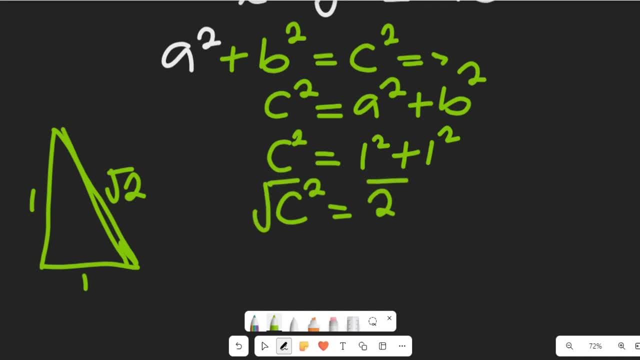 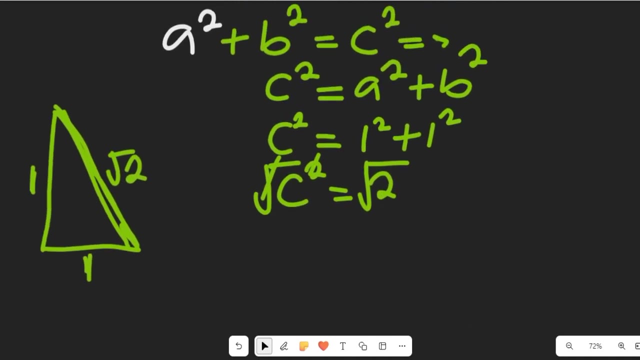 two and therefore take the square root of both sides. we're going to have c to be equal to square root of two. so the side we'll have is one one, and then square root of what two. that defines the size of the Pythagoras' Theorem. Now we're going to consider a Pythagoras' Theorem. 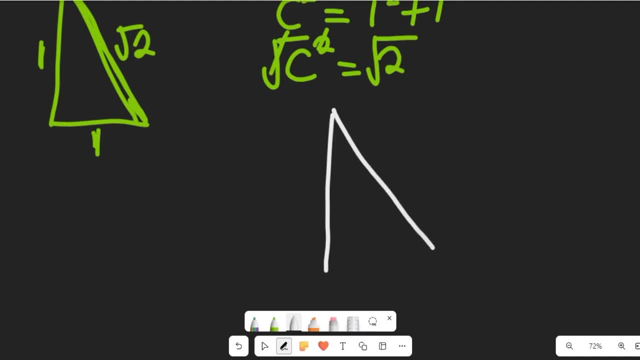 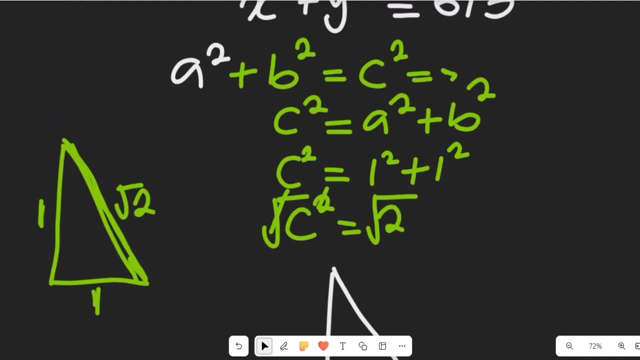 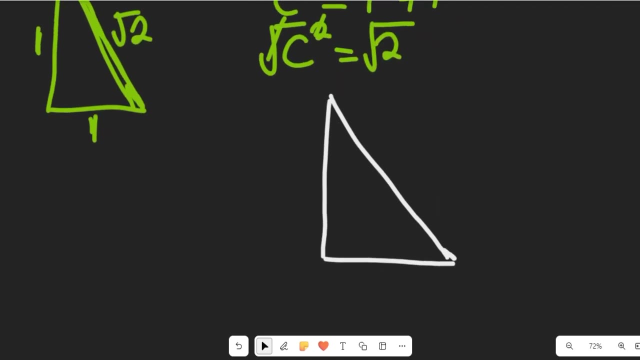 as we simplify this from the Pythagoras' Theorem you come to see that we're going to have these variables. we are given x, y and six, one, three. We're going to put them in inside them as p taking the place of e. so from here you can see. 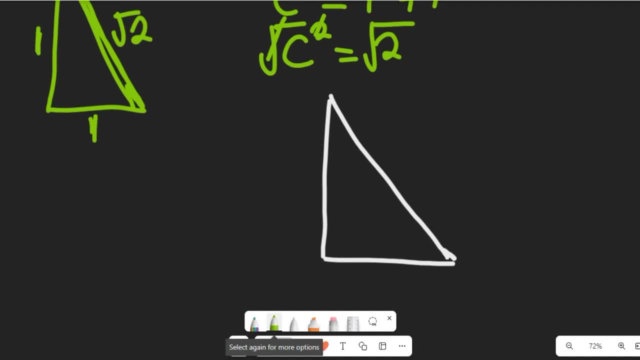 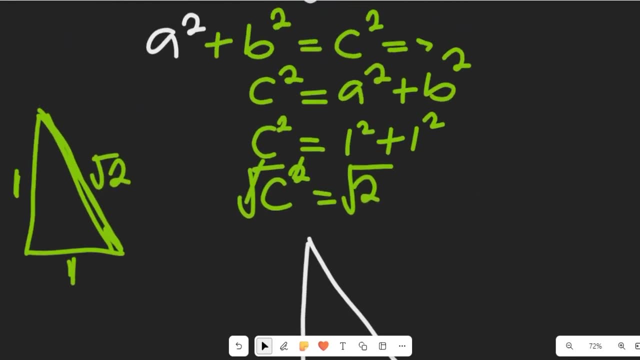 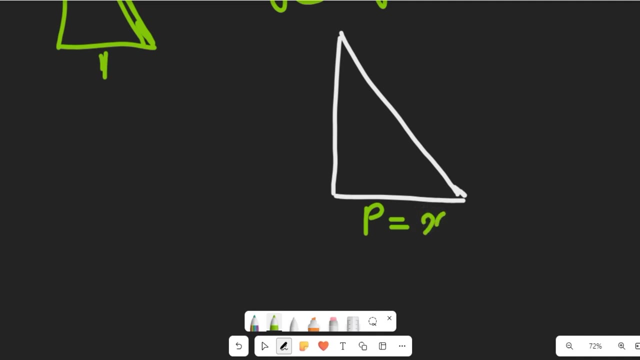 that if we apply that into that expression, you'll come to see that we'll take p to be equal to the first part, which is going to be x. p will be equal to x, so we'll take p to be equal to x. so if p is, 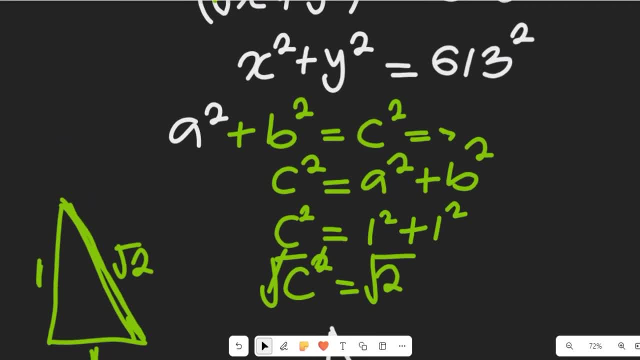 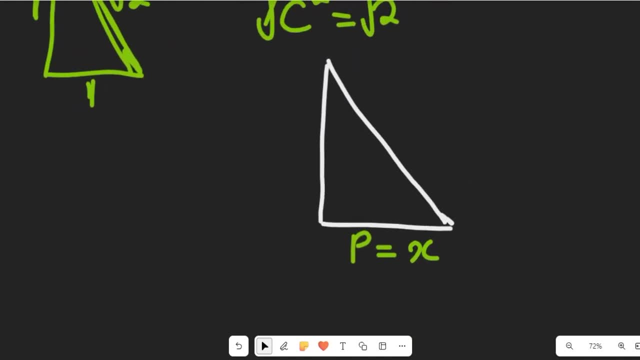 equal to x, which is the first part. that means we can be able to find y and six one three, and six one three represents the hypotenuse, so a six one three will be equal to a six one three, which is the hypotenuse. c is going to be represented with z, because we'll have z squared equal to. 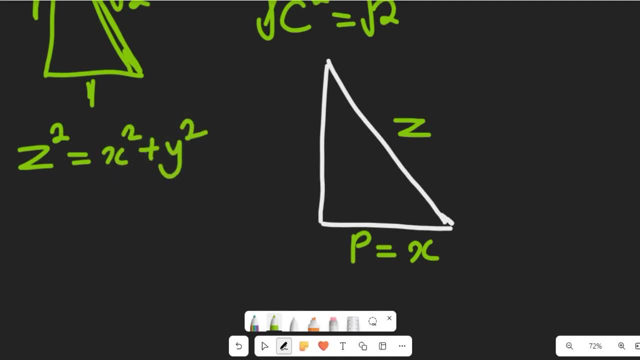 x squared plus y squared right, x squared x is equal to p, then z will be equal to six one, three right, and that will be equal to considering this whole part. you come to see that z will be equal to uh. if we have the first part, x, to be p squared plus if this part represented by one is equal to as z squared. 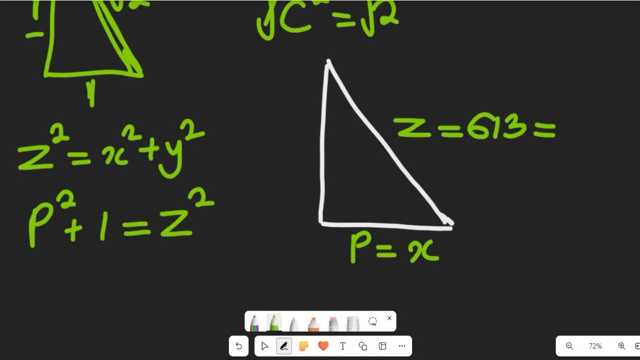 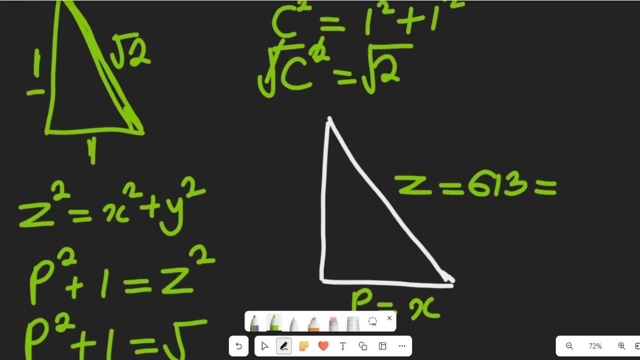 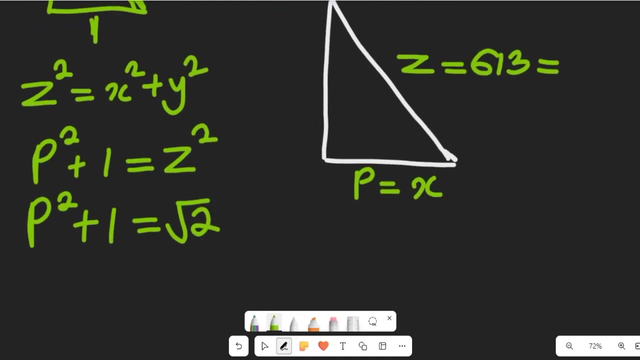 right. so if this, we divide this part by two, remember, as z squared is represented by d squared, plus one equal to is represented by the square root of two that we see over here. right, good, so we're going to consider that to be the square root of two. so if we take the 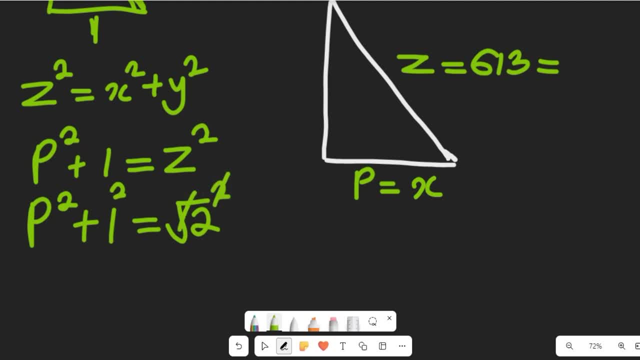 square of both sides, you'll come to see that this square will clear this square and will be left to it what t? squared plus one equal to two. so if we decide to divide both sides by two and divide both sides by two, we'll come to see that these sides will give us one which is still equal to z, and 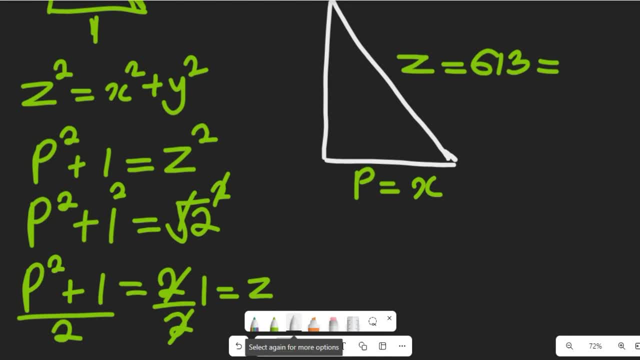 then the value of c will be t squared, that is, p squared plus one divided by two. now, if you check this other side, you see that our value of y, which is more like the, uh, the adjacent, this is the opposite of this angle, the opposite, this is the adjacent and this is the hypotenuse which is: 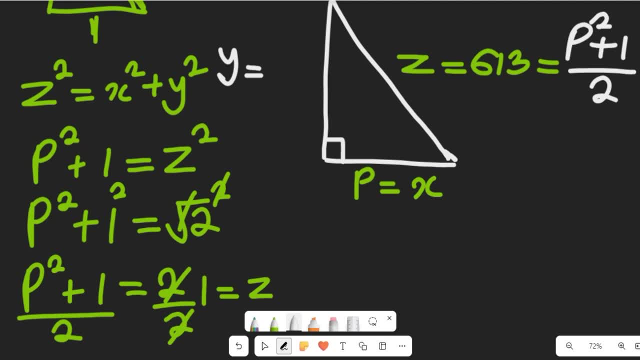 the- this is the hypotenuse. the z- this is the opposite of this angle. theta- this is the adjacent y. the longest side stands as the hypotenuse. so this is going to be p squared minus 1 divided by 2, because it is the opposite side. so from this part we can see that the value of 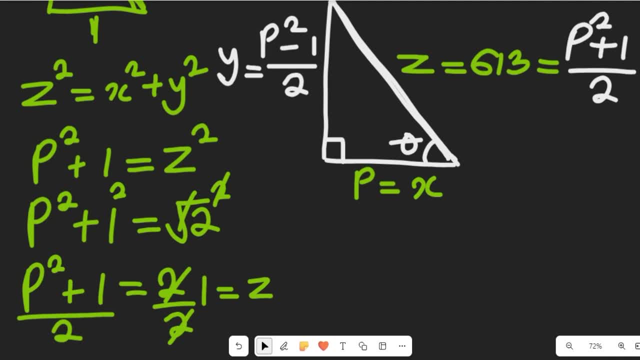 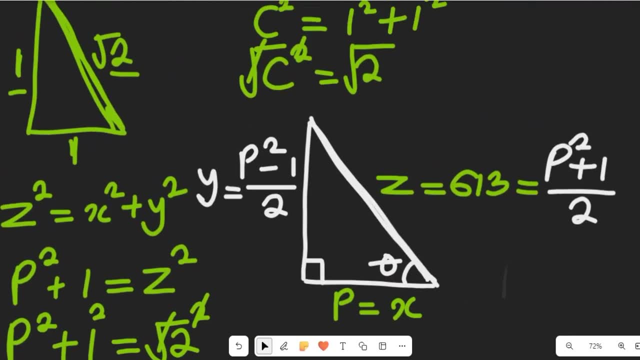 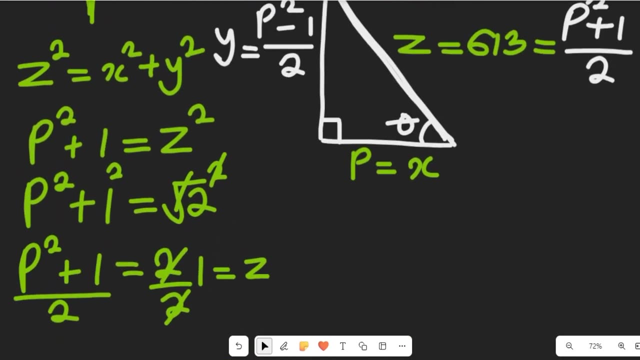 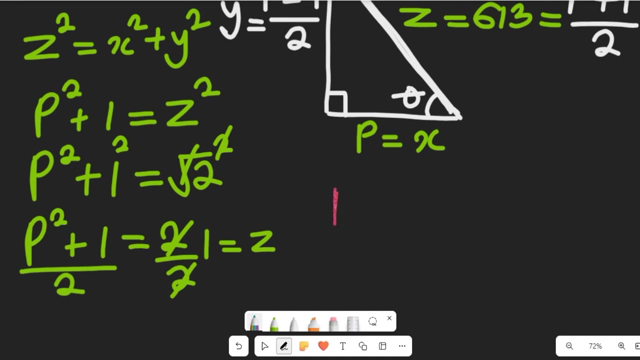 x, y and z are being replaced with the letter p, so from here we can simply simplify this expression. from this expression now we can see that our x square plus y square is equal to 6, 1, 3. so from the values of x and y itself we can get the value of value of p, because there we have that p squared. 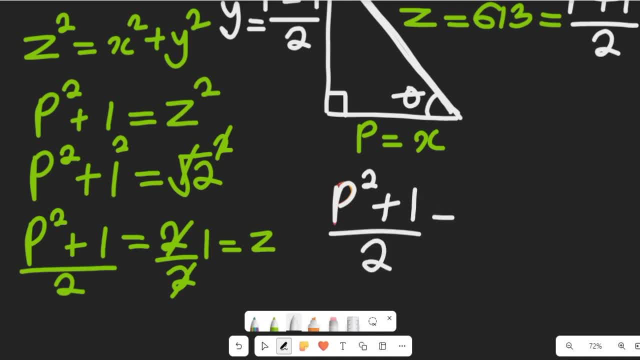 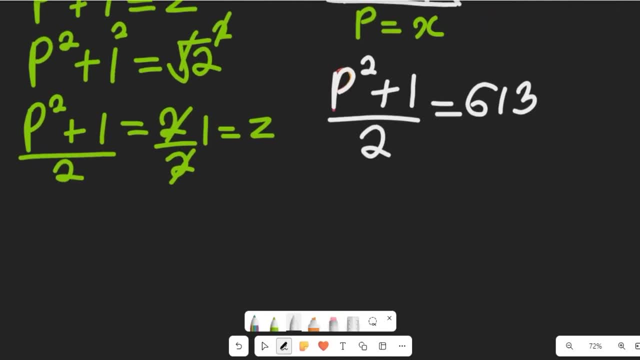 right plus 1 divided by 2 is equal to 6 1- 3. so from this expression we can simply find the value of p, and the value of p will be equal to p square plus 1, equal to 6 1- 3 multiplied by 2.. so our p squared will be equal to. 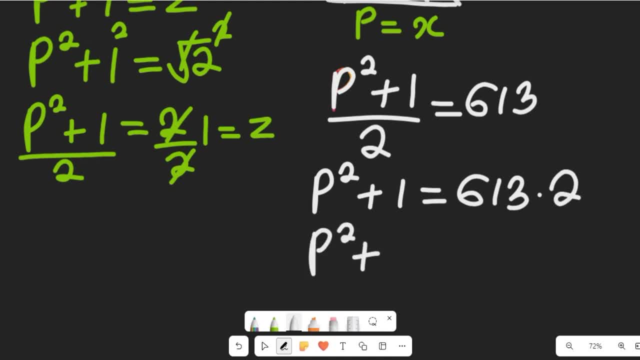 3, 1 plus 1 will be equal to 6. 1. 3 multiplied by 2 is going to simply give us 6 times 3 will give us 6, that will give us 6, 2, and 6 times 2 will give us 12. so the value of our p will be equal to. 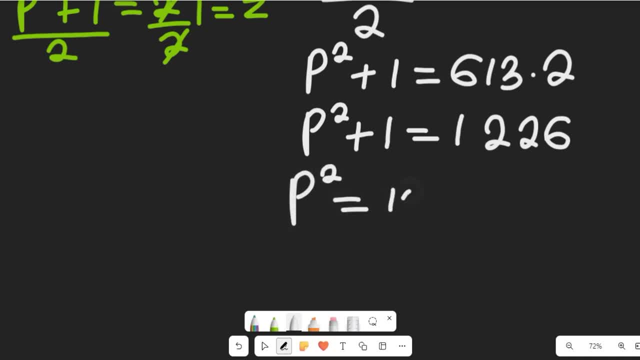 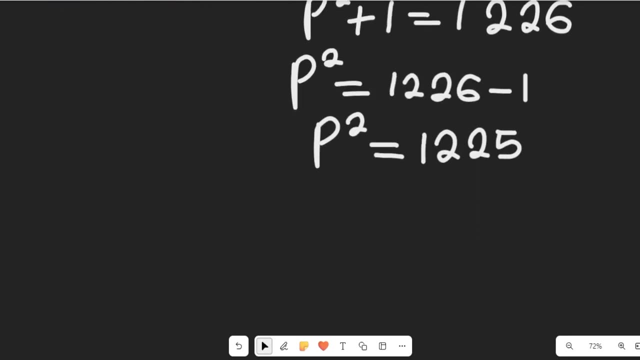 p squared will be equal to 1, 2, 2, 6 minus 1, and then our p squared can now be equal to 1, 2, 2, 5. now to find the value of p, we are simply going to take the square root of both sides, so we'll have: 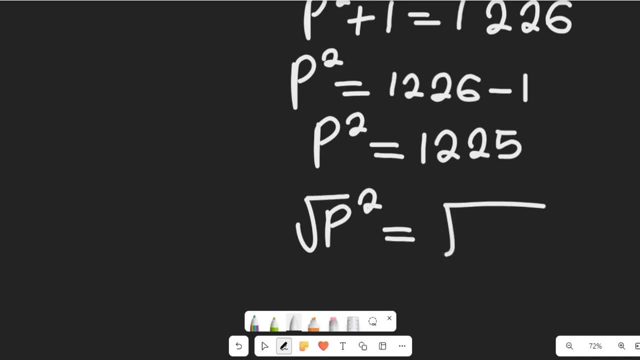 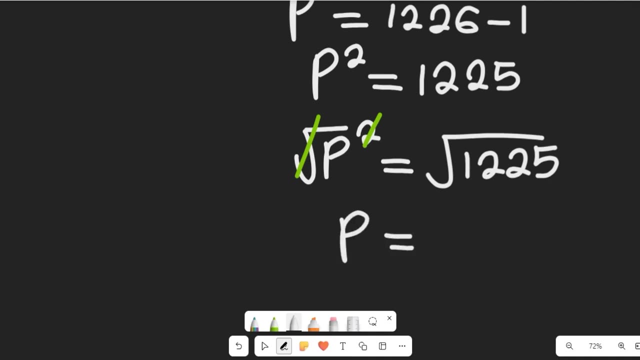 p squared to be equal to the square root of 1, 2, 2, 5, and what will this give us? this is going to clear this, and then the value of our P will be equal to. P will be equal to the square root of 12. 25 is going to give us 35, because square root. 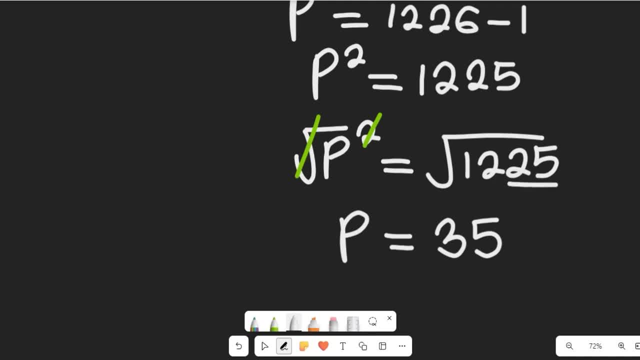 of 25 is 5 and the square root of 12. to simplify, it is going to give us 4 times 3, which is equal to 3, so the value of our P will be $35. so which, true, have gotten the value of our P to be a whole 235 from the. 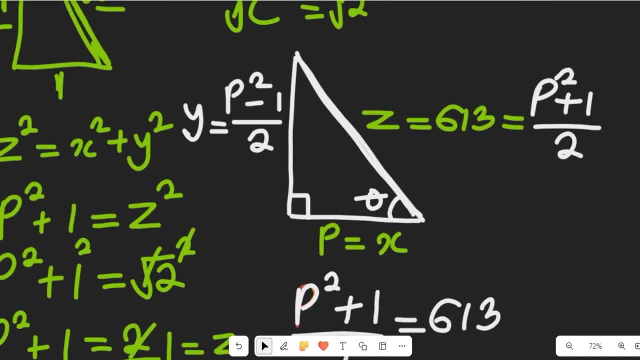 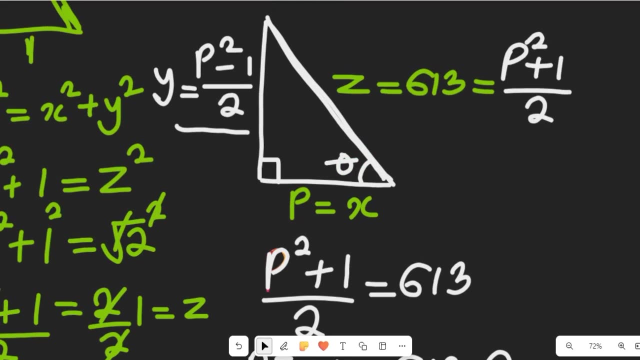 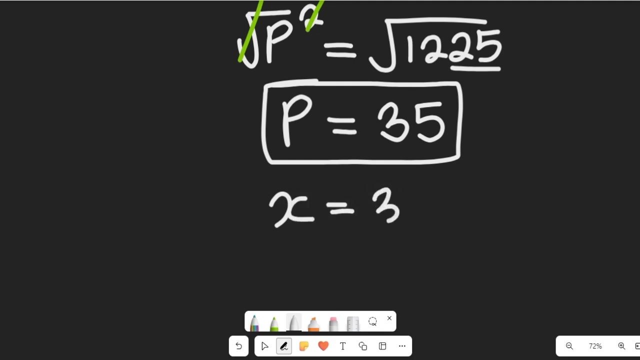 expression on that Pythagoras theorem or kind final, that we can easily find the value of Y. from here we can sign: we find value of Y because the value of our P is equal to 35 and recall that our P, p is equal to x. so the value of x simply is equal to 35. so if we find the value of x, we 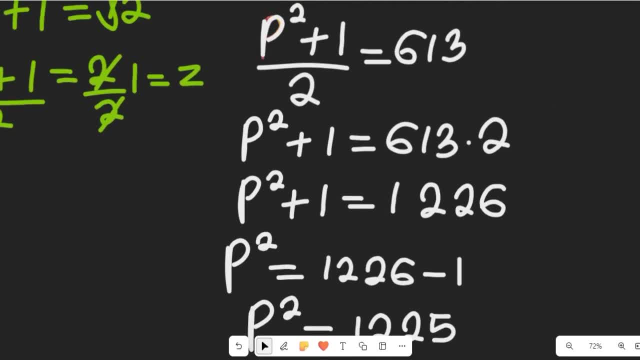 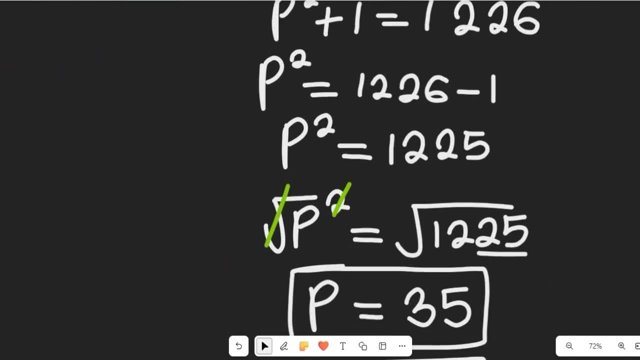 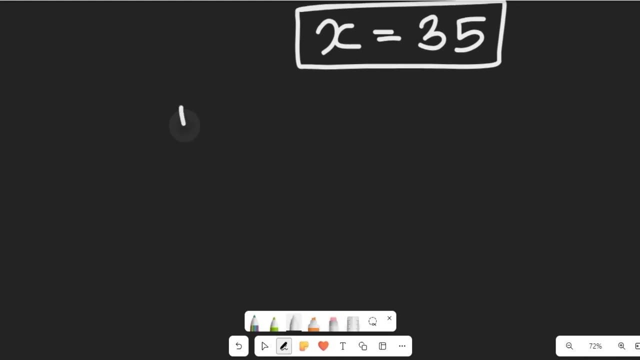 can simply find the value of y using the opposite of that triangle. if we find the opposite of that isosceles triangle, we're going to see that this is going to give us, this is going to give us y equal to p square minus 1 divided by 2. so for half this, the value of p being 35. 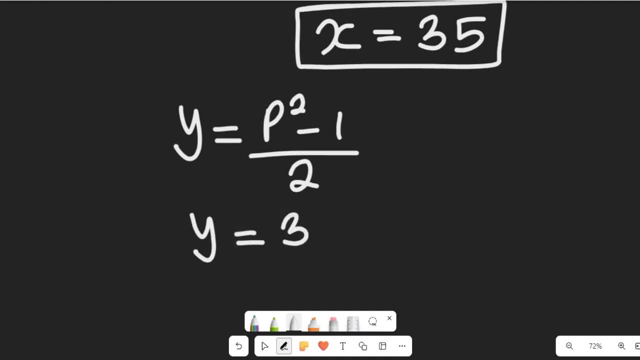 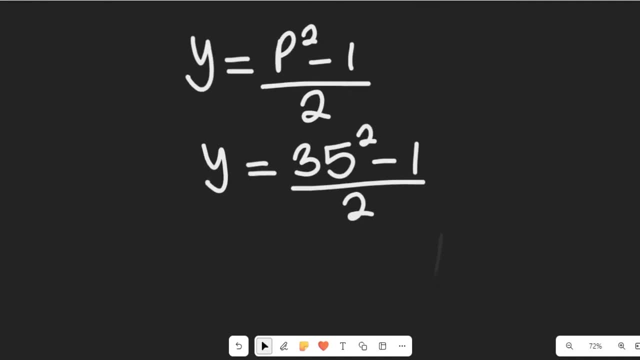 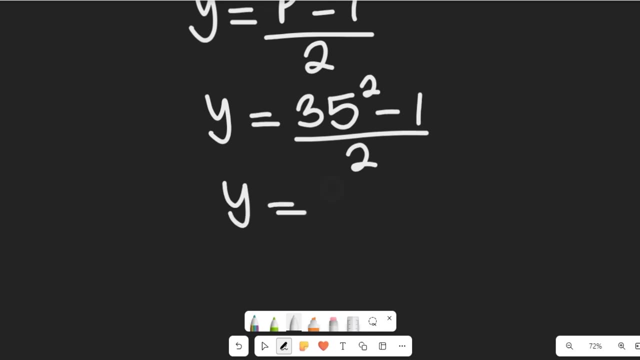 then our y will be equal to 35 square minus 1 divided by 2. so 35 square is going to give us our y will be equal to the square root of 35, will give us 1, 2, 1, 2, 2, 5 minus 1, and this will be divided by 2.. 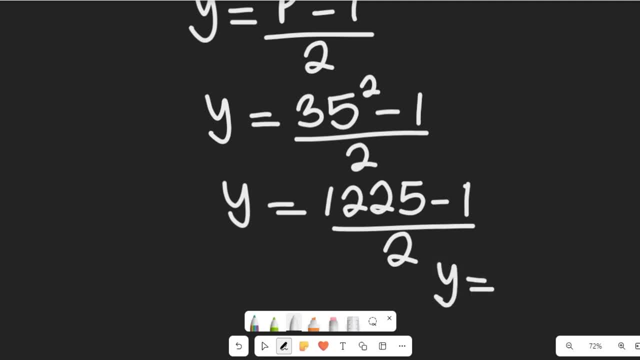 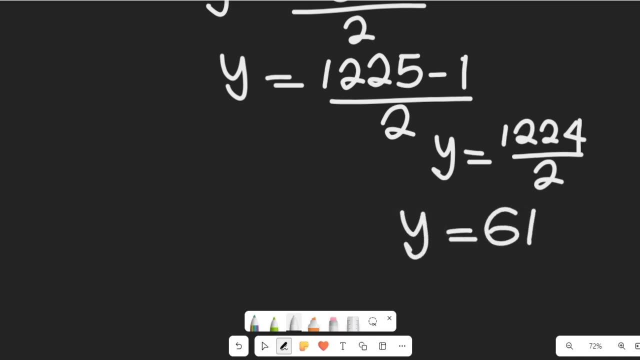 So the value of our y will be equal to 1,, 2,, 2, 4 divided by 2.. So our y will simply be equal to: this will give us 6,, this will give us 1 and this will give us 2.. 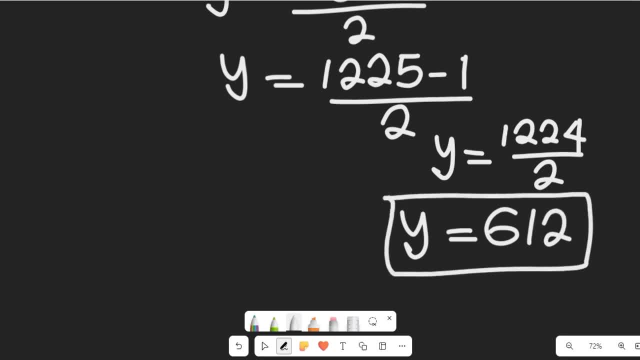 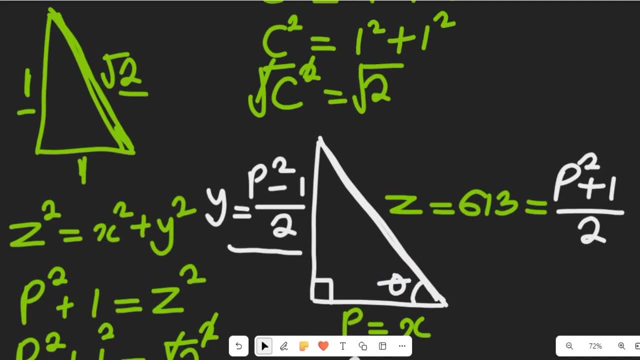 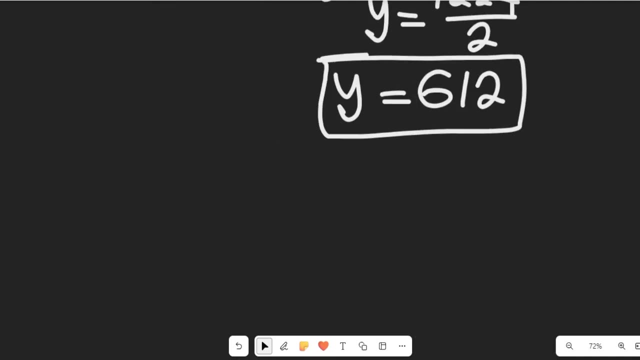 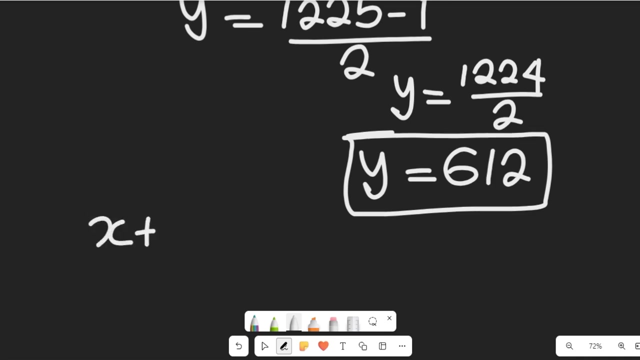 So our y will be equal to 6, 1, 2.. Now, from the initial expression, we are asked to find the value of x plus y, right? So we're going to look for the value of x plus y. The value of x plus y is now going to give us. the value of our x plus y will now be equal to 35.. 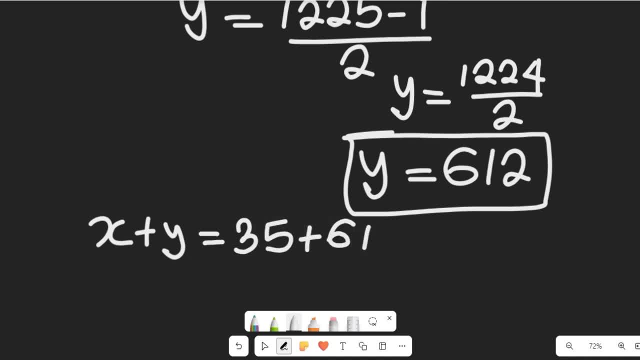 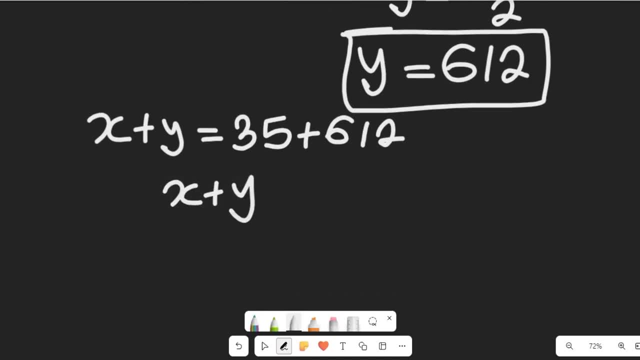 35 plus 6, 1, 2 and 35 plus 6, 1, 2, then our x plus y will be equal to. this is going to give me 7.. 5 plus 2 is 7, and this will give me 4 and then 6.. 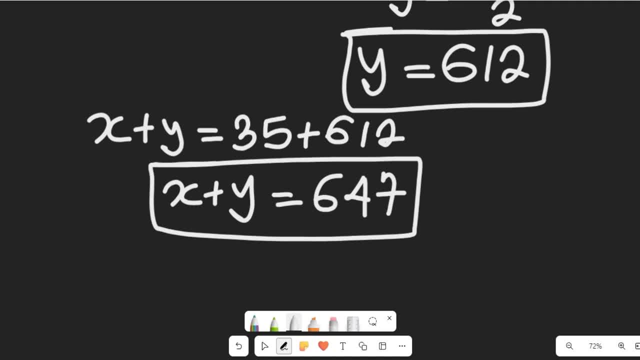 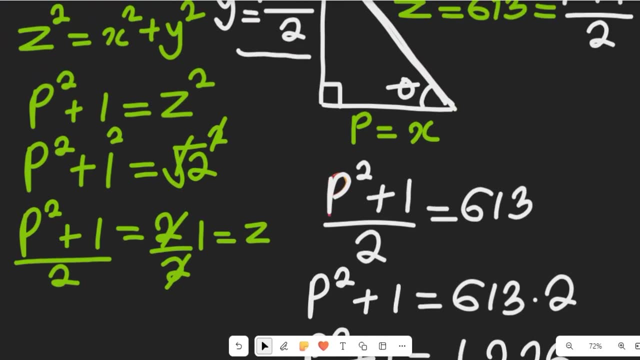 So the value of x plus y that satisfies that question given to us is 6,, 4, 7.. Now it's going to be interesting if we can check if this expression or the solution we get is absolutely correct. Now let's check. 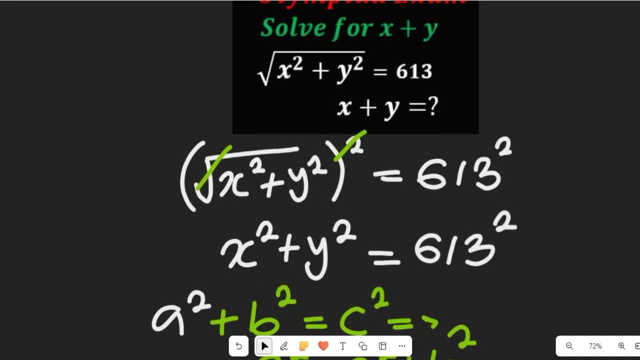 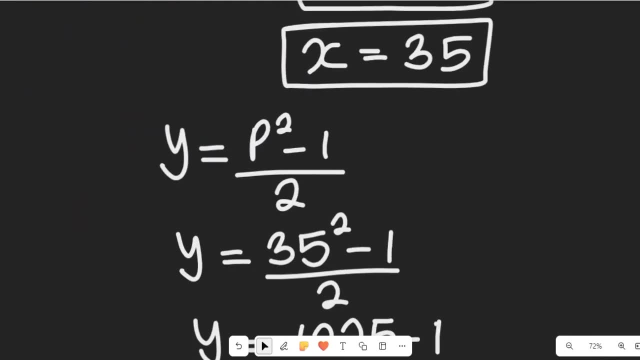 From the initial expression we are given that x squared plus y squared, the square root of x squared plus y squared, should be equal to 6, 1, 3.. Now let's check that to find out if that expression is actually correct. 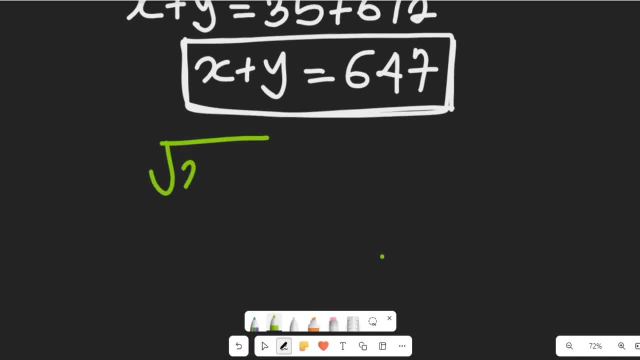 We are given the square root of x squared Plus y squared to be equal to 6, 1, 3.. With the value of our x equal to 35 and the value of our y equal to 6, 1, 2.. 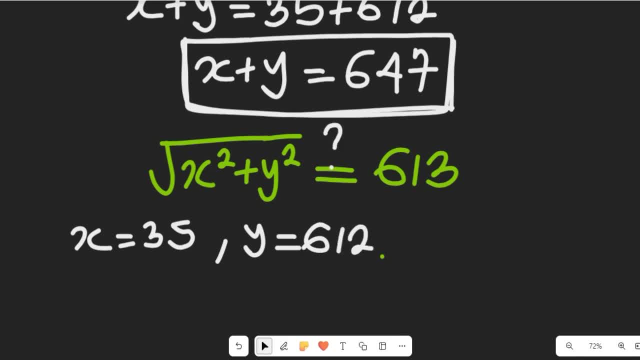 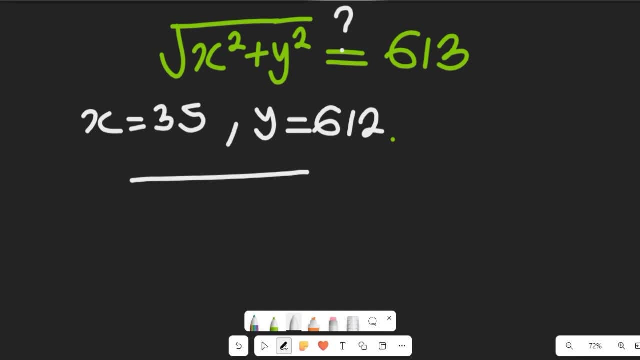 Can we get 6, 1, 3 as the square root of the square of these two values? Let's find out. Let's find out. We are going to have the square root of 35 squared, plus the square root of 6, 1, 2 squared is equal to give us 6, 1, 3.. 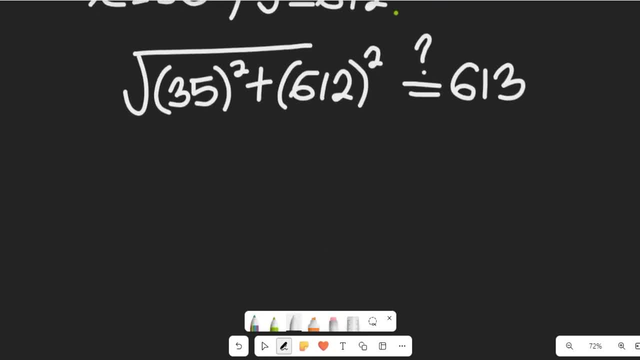 Now let's simplify that. The square root of 3, 5, that is, 35, is going to give us 1, 2, 2, 5.. Plus, the square root of 6, 1, 2 is going to give us 3,, 7, 7, 5.. The square root of 6, 1, 2 is going to give us another 3, 5,, that is 35,, that is 35,, that is 42.. So the square root of 6, 1, 2 is going to give us 5, 6, 5..